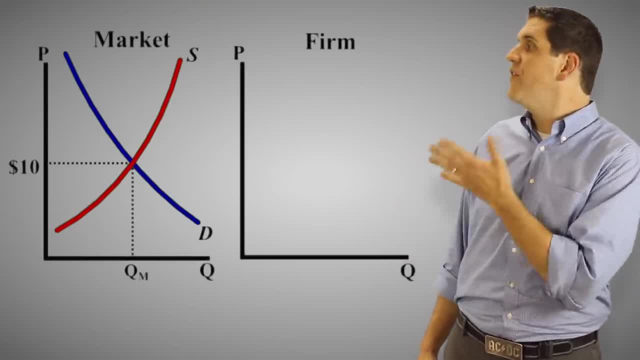 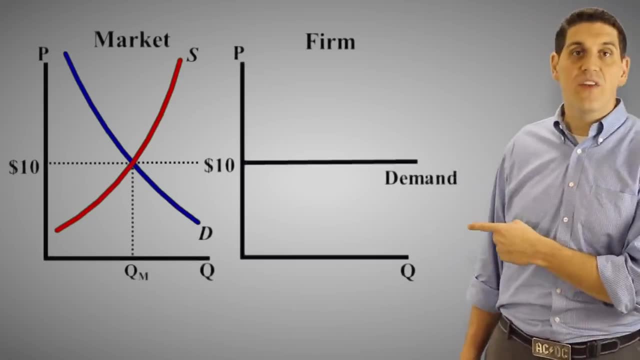 So this is the industry graph, or the market graph that includes all the different firms that produce milk. Right here is the graph for one individual firm, And since they're price takers, the demand for this firm is horizontal. It's perfectly elastic. Again, this is because they have no. 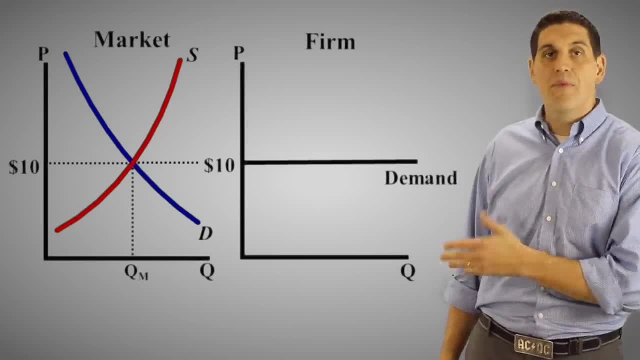 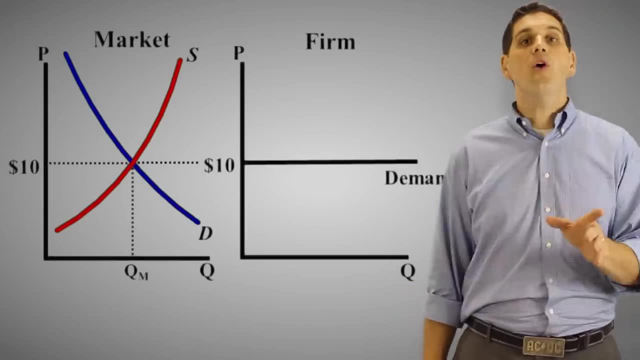 control over the price. If they raise the price up to 11, then no one's going to go to them. They'll go to all the other dairy farmers And there's no reason for them to lower the price below 10, because people are going to buy as many units as they sell at $10.. This horizontal demand curve is 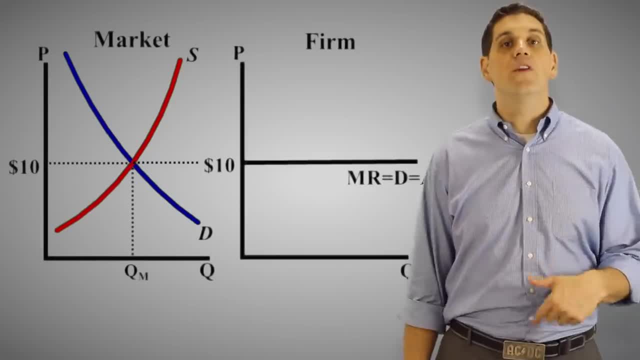 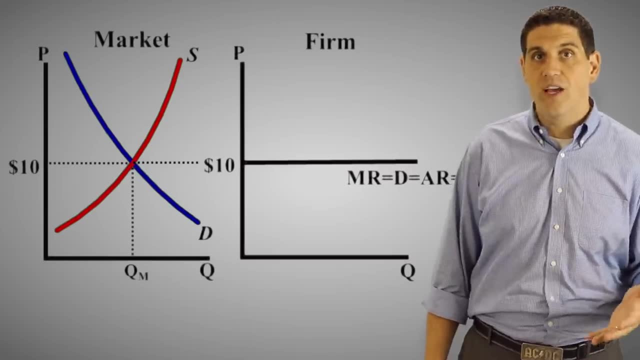 the demand, but it's also equal to the marginal revenue. Marginal revenue is the additional revenue that the firm gets when they sell another unit. So if they sell another crate for $10, their additional revenue is $10.. They sell another crate for another. 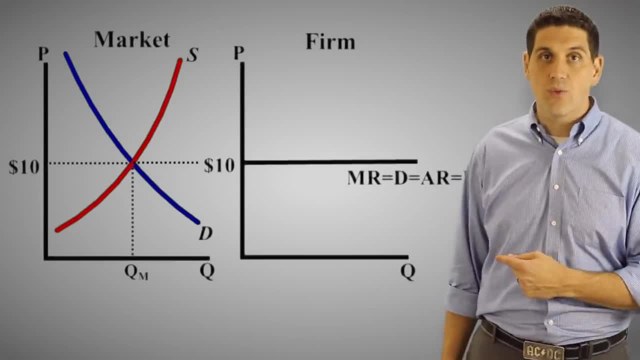 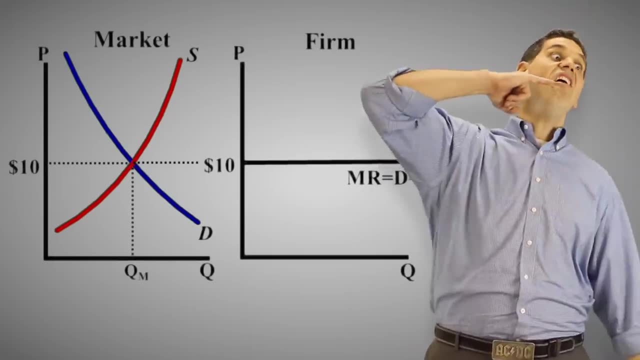 $10, additional revenue $10.. So the demand equals the marginal revenue. It also equals the average revenue and the price, And your teacher will probably tell you this is sometimes called Mr Dart. That's something I do in my classes. Anytime I say the word Mr Dart, the students 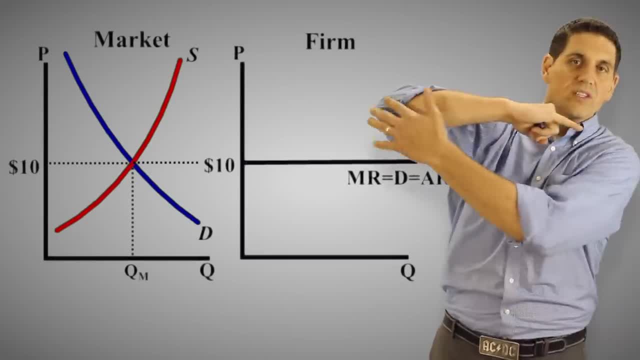 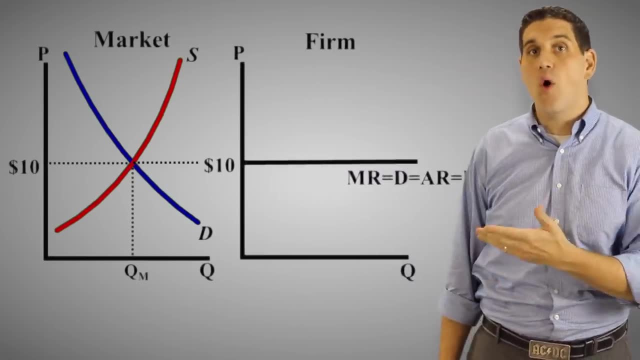 have to go. This is the horizontal demand curve, which equals the marginal revenue. The point is, the demand and the marginal revenue are horizontal for the firm. Now if we take some cost curves and put it on here, we can actually figure out how many units this firm should produce. 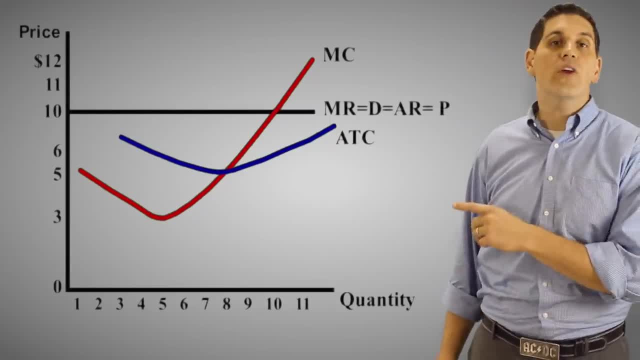 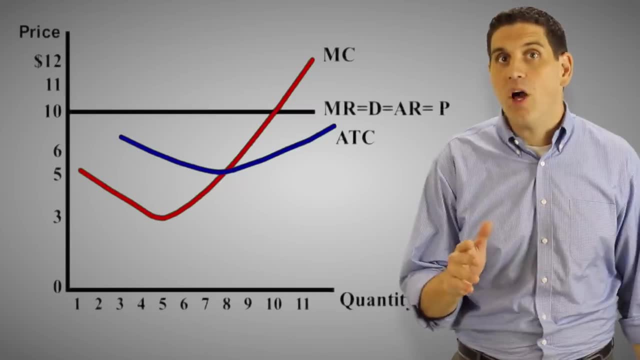 and we can calculate profit. So let's zoom in on the firm Notice. we have a marginal cost curve and an ATC. The first question is to figure out how many units they should produce. Well, that brings up the most important concept in all of microeconomics, which is the profit. 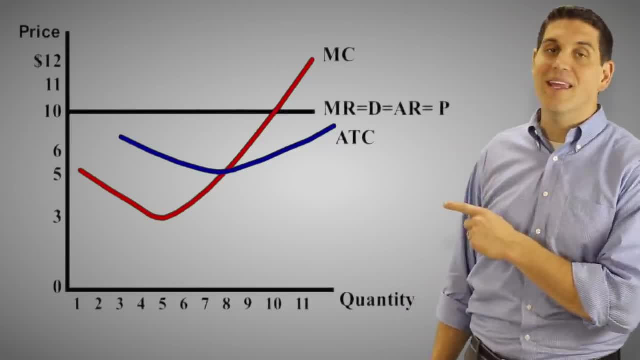 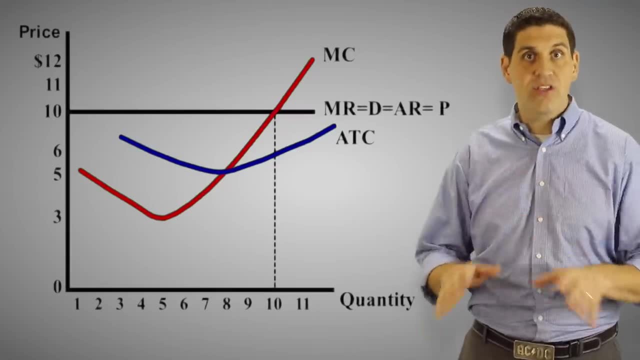 maximizing rule. All firms should produce where MR equals MC. This is basically saying the profit maximizing rule is that you should always produce as long as the marginal revenue is greater than the marginal cost. At the point where they're equal, you should stop producing, and that's the profit maximizing quantity. If you produce where the marginal 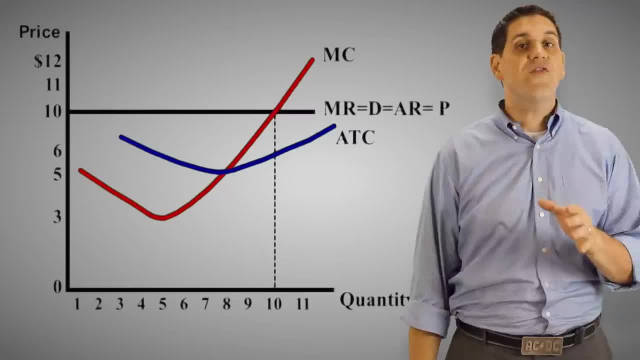 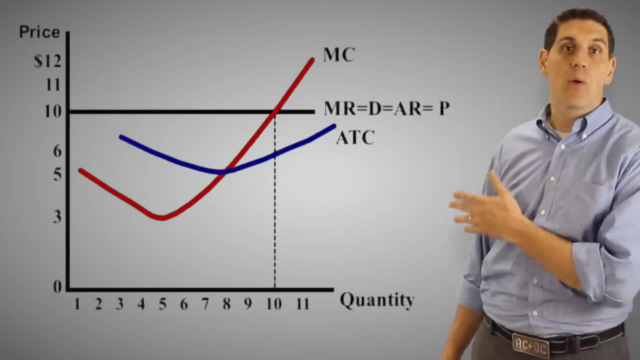 cost is greater than the marginal revenue, you're going to make less profit than before. This firm is going to produce where MR hits MC, which is right there, at 10 units. They don't want to stop at four units because they can still produce more profit, And they don't. 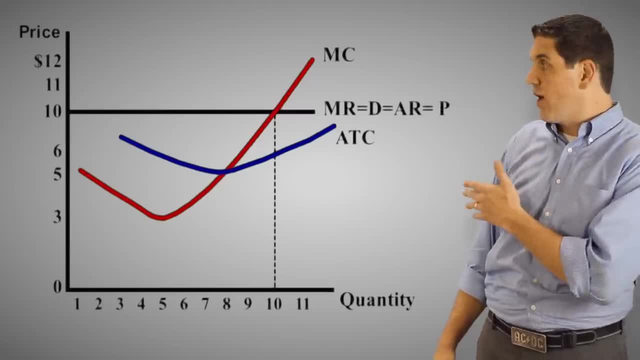 want to produce 11 units because the additional cost is greater than the additional revenue selling that unit. This is why you spent so much time learning about all the cost curves. You put them together with the revenue curves and now you can figure out how many units you're going to produce.